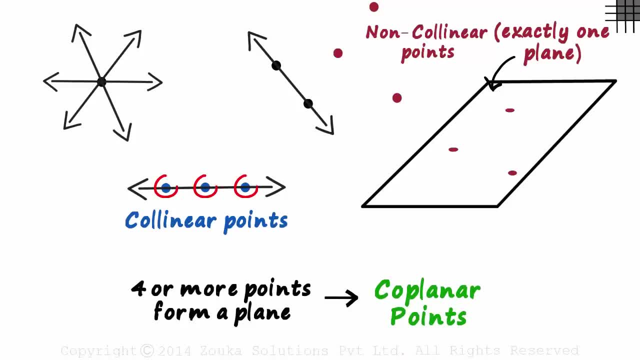 Understand these concepts well. Three points are co-linear. if exactly one line passes through them, Exactly one plane passes through three non-co-linear points, And if four or more points form a plane, they are called co-planar. Co-planar is basically one plane. 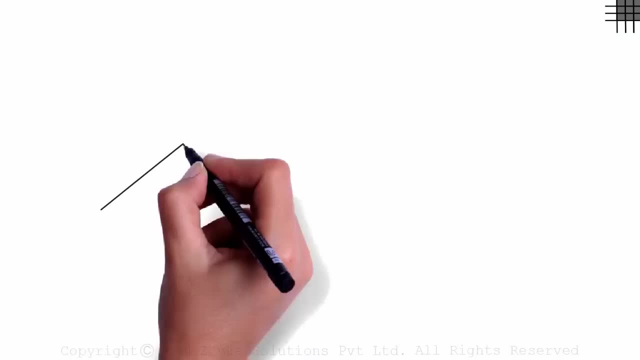 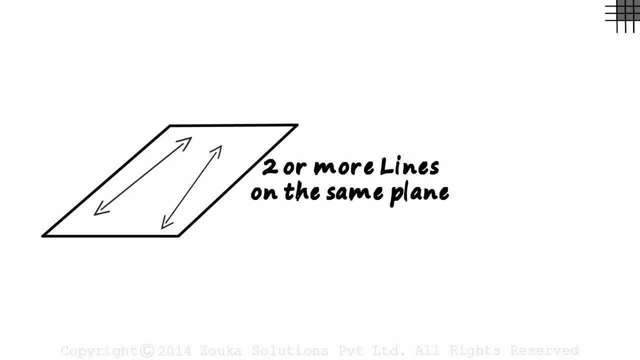 So when are two or more lines co-planar? Easy: if the lines lie on one plane, they are co-planar. Two or more lines lying on the same plane are called co-planar lines. When are two lines not co-planar? 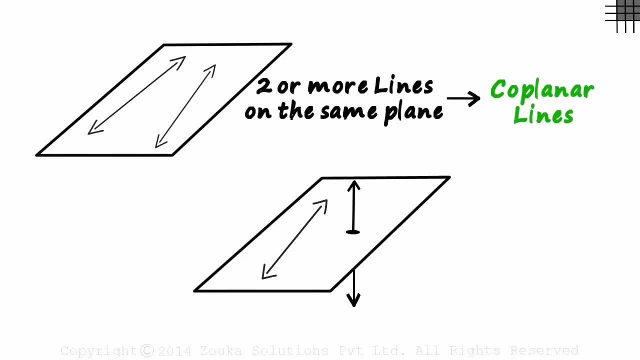 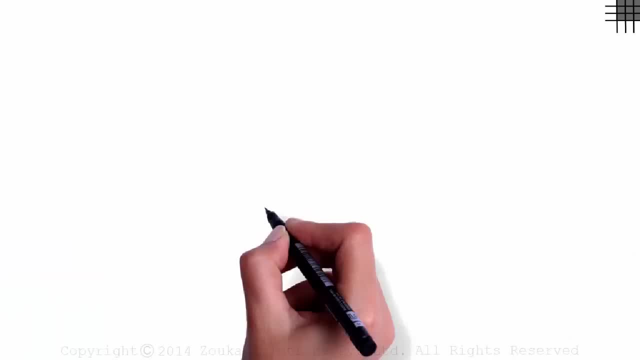 If two lines do not lie on the same plane like this, then they are non-co-planar. And we look at one last combination of a line and a point. Will they lie on one plane? Yes, a line and a point will always lie on a plane. 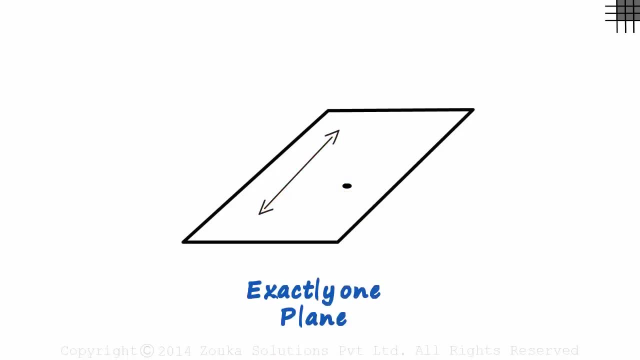 exactly one plane. It doesn't matter how you position the point or the line. You can move them both as you wish. You will always have one plane passing through them. 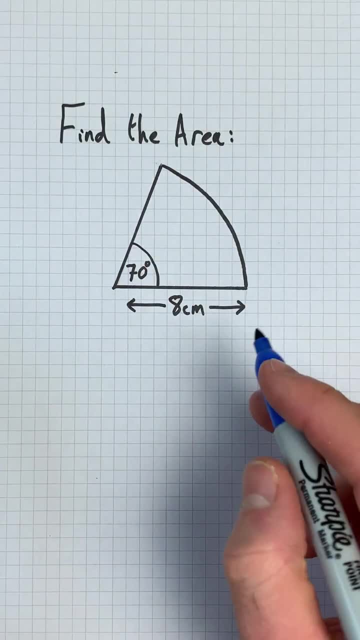 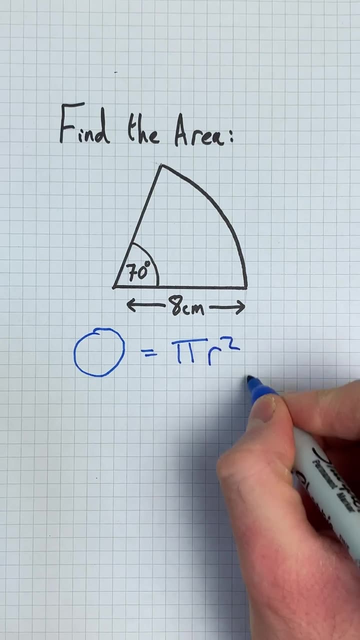 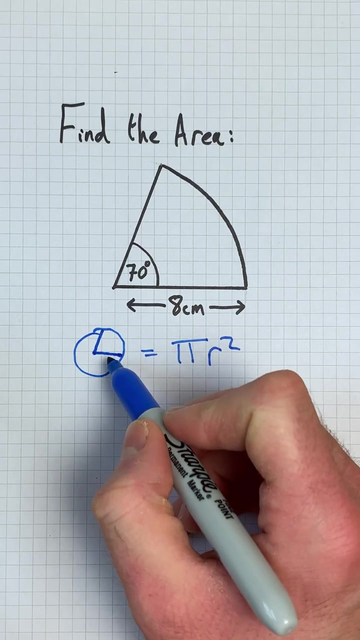 Here's how you find the area of a sector. The first thing you need to know is that you can find the area of a full circle by calculating pi multiplied by the radius squared. This means that if you want to find the area of a section of this circle, what you need to do is multiply. 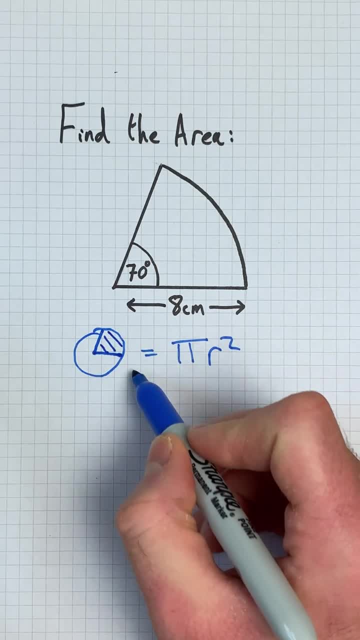 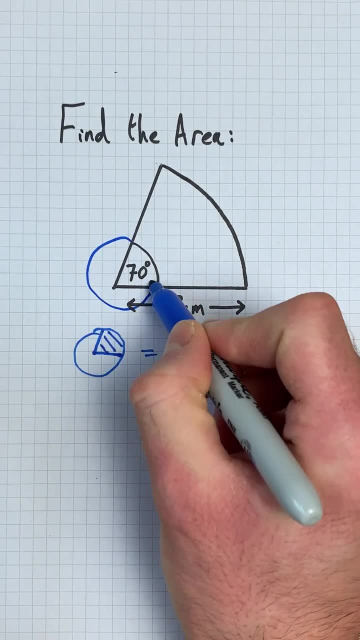 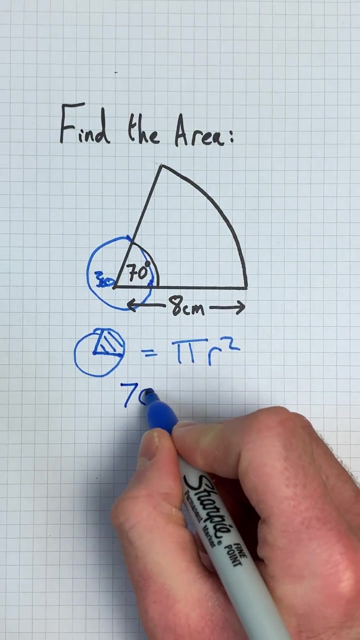 the fraction of the circle's area taken up by this sector. by pi r squared. In this case, you can see that the angle we have is 70 degrees and in one full circle there are 360 degrees. This means that the sector we have here is 70 over 360 of a full circle. This is the fraction. 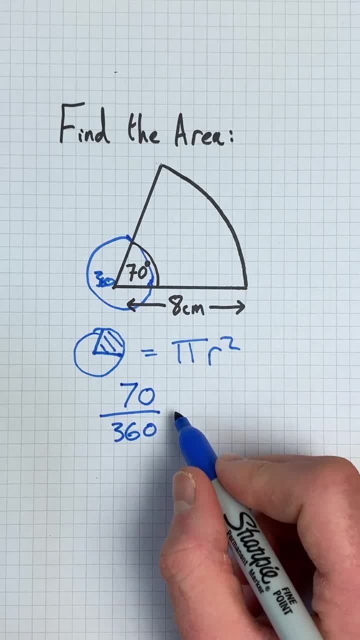 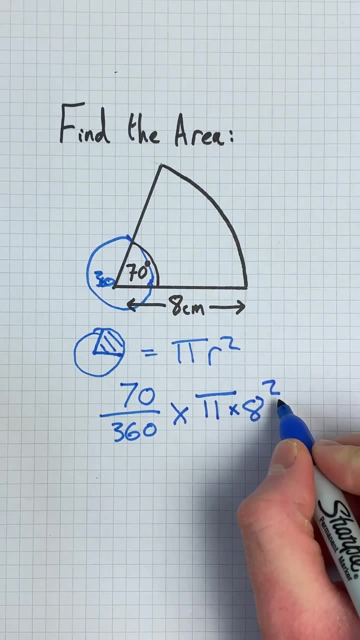 of the circle's area taken up by this sector. So, then, all we need to do is multiply this fraction by pi times by the radius squared. If you enter this in on your calculator, you should get a value of approximately 39 centimeters.